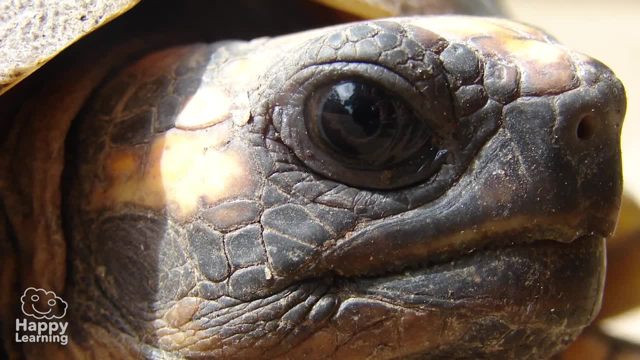 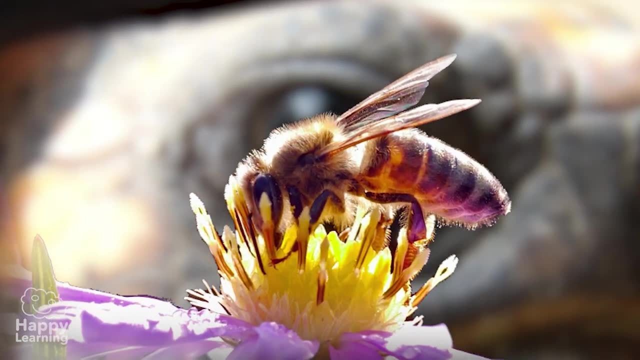 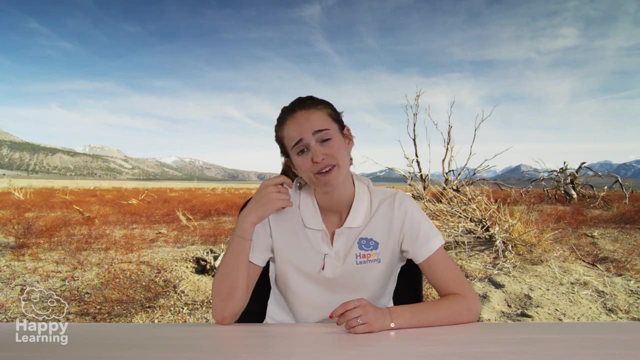 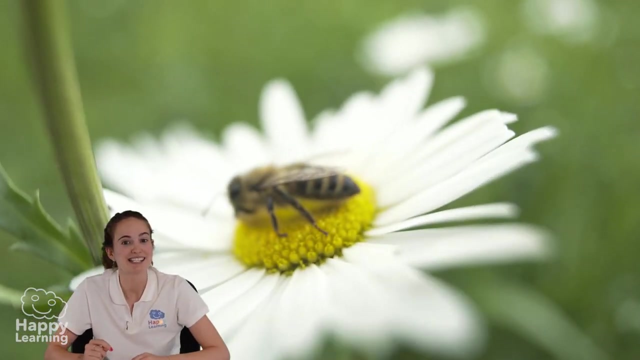 polar bears, Tortoises, Even bees, are close to being extinct. Actually, in some places they have already disappeared completely, and that makes me sad, very sad. But do you know how we can help the animals? The first thing we need to do is learn lots of things about them. Where? 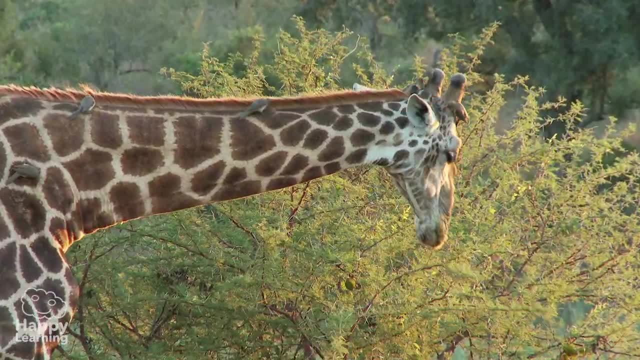 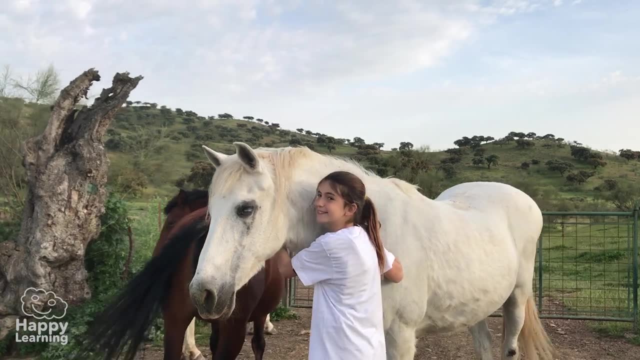 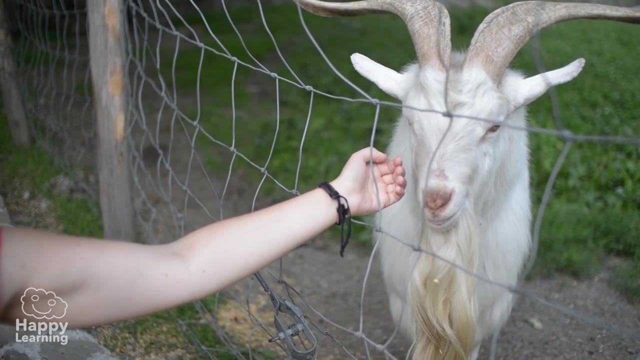 they live, What they eat, What they eat And how they are affected by what us humans do. The more we know about animals, the more we will love them, because they are so great and so beautiful. Also, some of them are so. 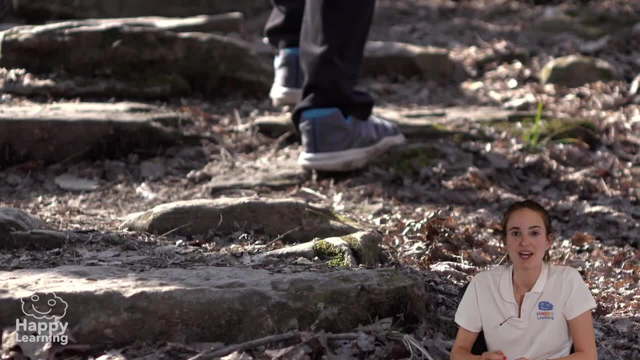 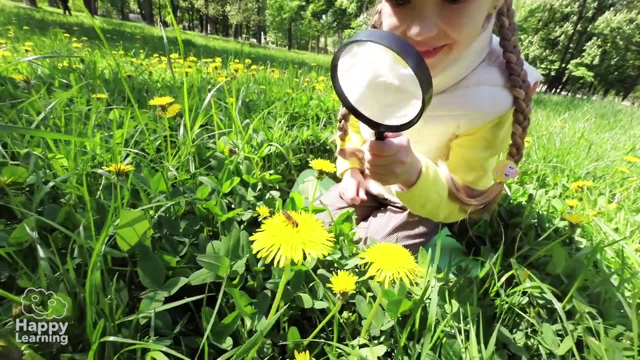 much fun. We should also take walks in the woods so we can get to know nature better. This way, we will enjoy it and take care of it like nature deserves. If I threw this stone at you, would you take it with you? No, I wouldn't take it with me. No, I wouldn't take it with me. 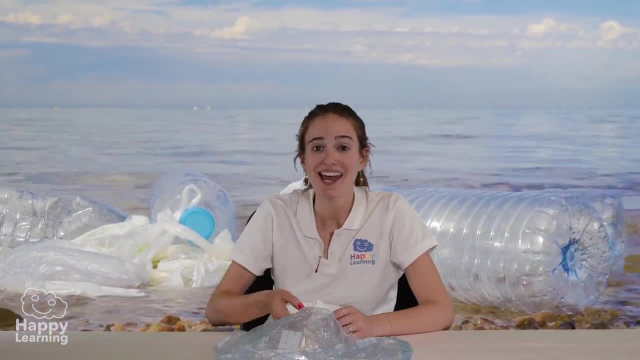 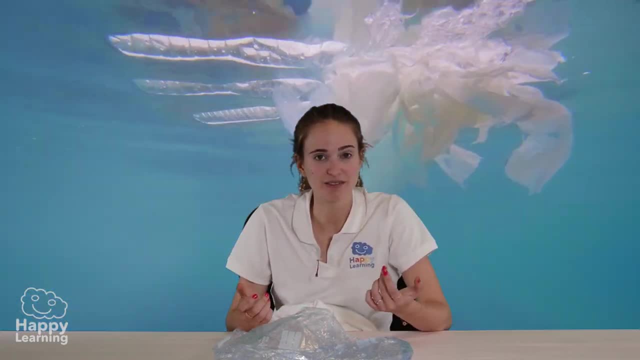 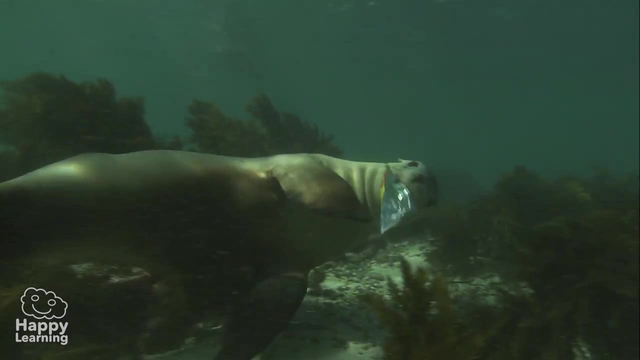 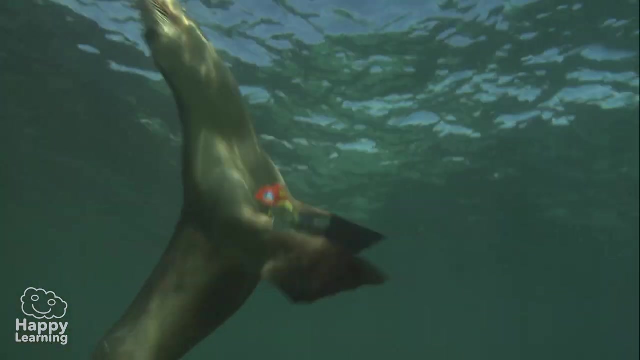 SEA CREATURE LIKE A DOLPHIN OR A SEA TURTLE. LOOK AT THESE IMAGES. This seal has eaten plastic, thinking it was food. Sadly, the poor thing will probably die. Do you realise how important it is to take care of nature? Another way of taking care. 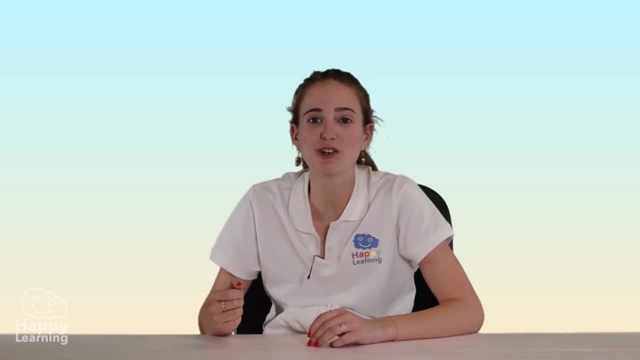 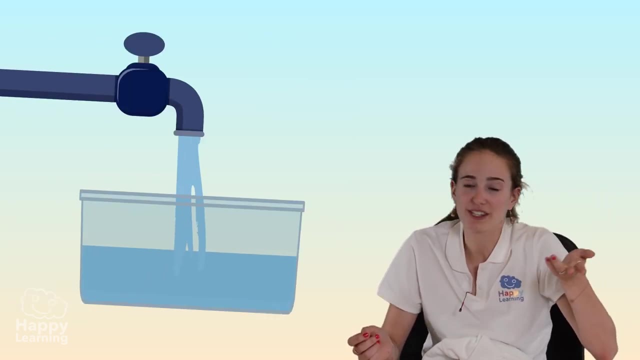 of nature and animals is consuming. What is the convenience of taking care of nature? For us, taking care of nature is not consuming in an ecological manner. and it's easy peasy: We can switch off lights when we aren't using them, turning off the tap or switching off the TV when we're not watching. 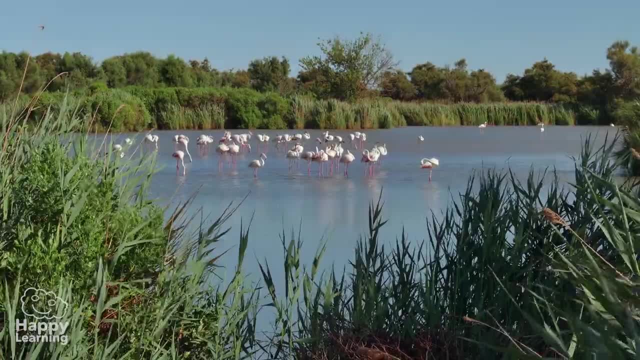 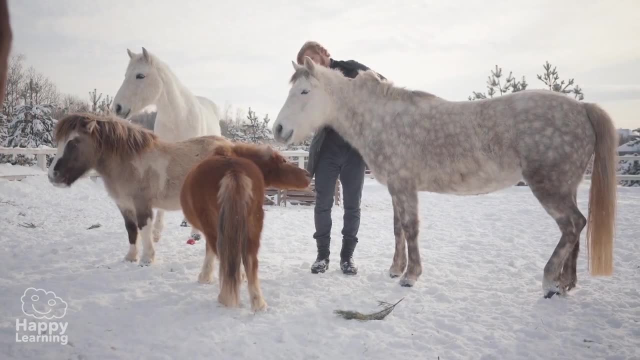 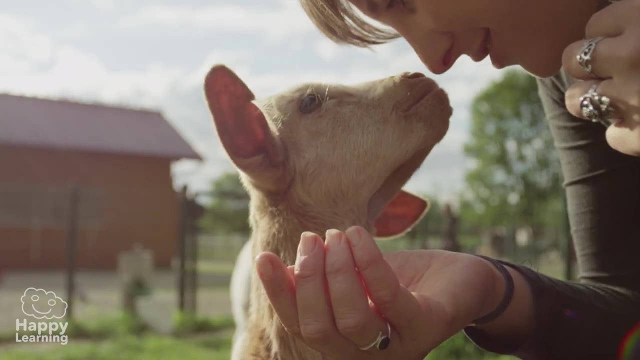 it, And if we all do these things, then nature will be a lot cleaner and animals will live longer and better lives, and they will never ever become extinct. We all fit in this world. the Earth is our home, but it's also the home to all other living things, So will you help? 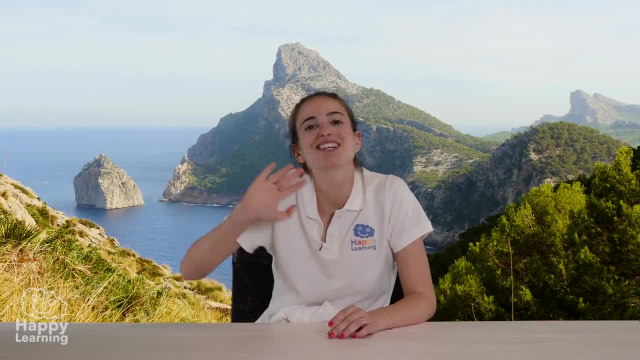 us take care of it. I hope you do. Goodbye, happy friends. I hope you're always ready to learn and taking care of the planet. Goodbye.